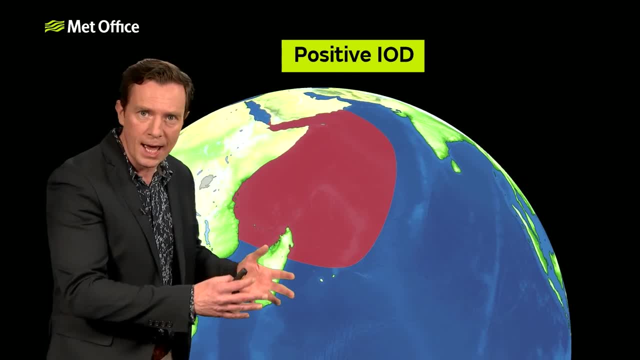 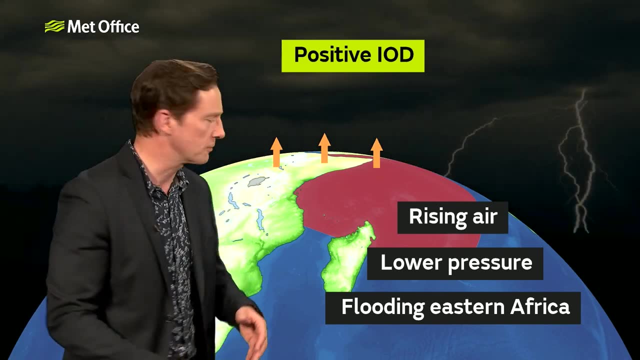 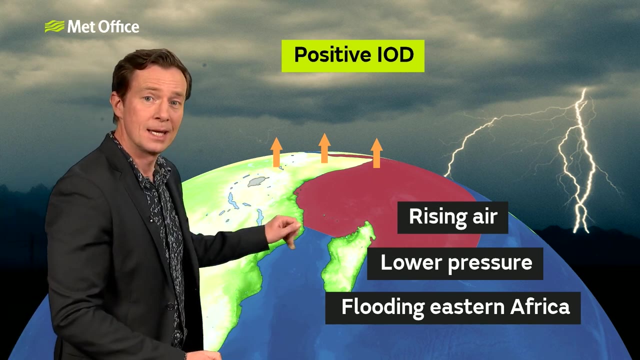 The higher temperatures over the ocean creates warmer air above the surface. That warmer air rises, That lowers the pressure at the surface, And the combination of low pressure and rising warm air generates more rain in this part of the world. Now it's not just here that's impacted. the whole ocean is. 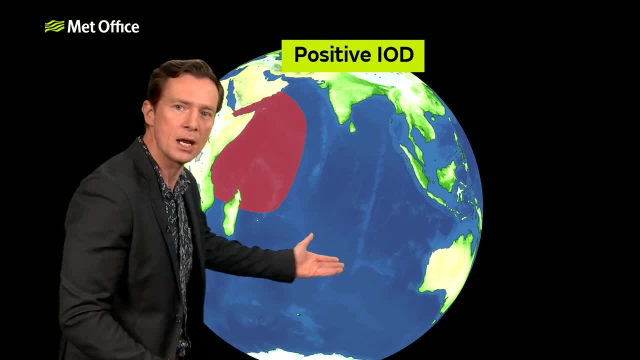 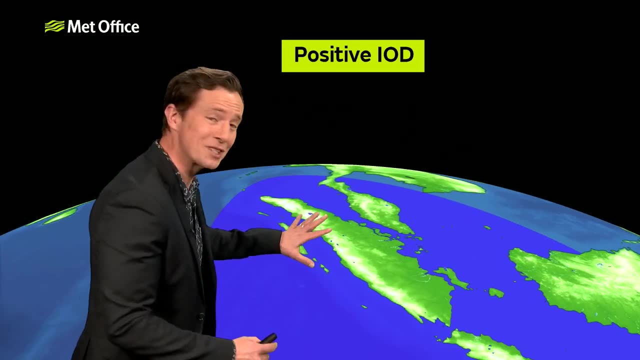 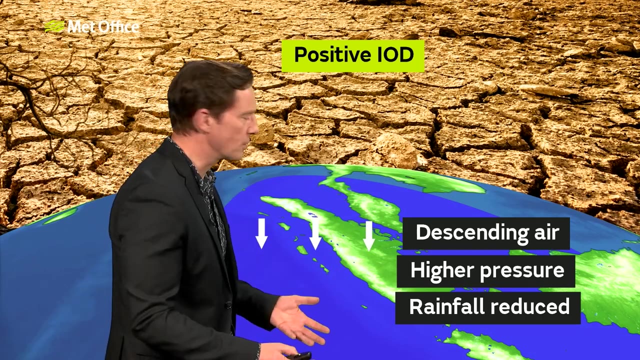 And as well as warming of the waters on the western side, an upwelling of cooler waters on the eastern side of the ocean is created at the same time, And the cooler waters here means that the air doesn't rise as much. pressure is higher at the surface and rainfall is reduced and droughts can occur. 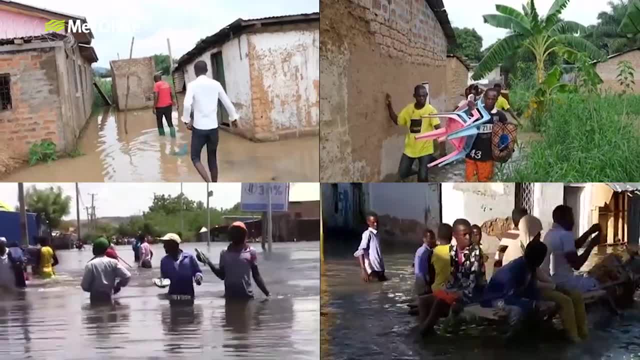 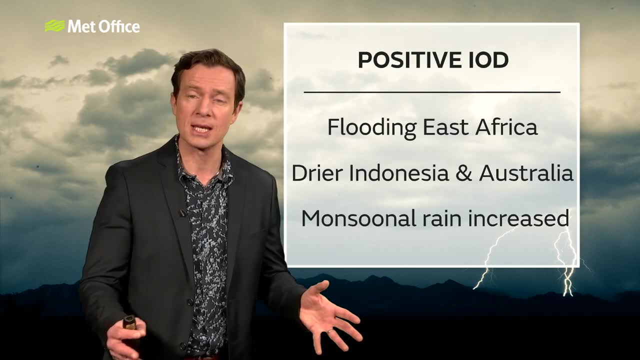 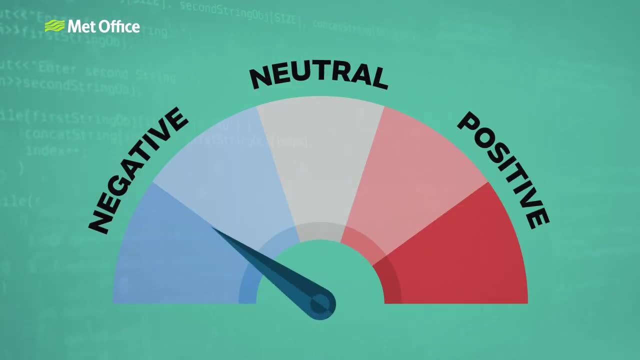 So when the IOD is positive, it usually creates flooding in eastern Africa and drought in Indonesia and Australia. A positive IOD also leads to an increase in rainfall during the southwest monsoon season across the Indian subcontinent. Now let's look at what happens when we get a negative IOD. 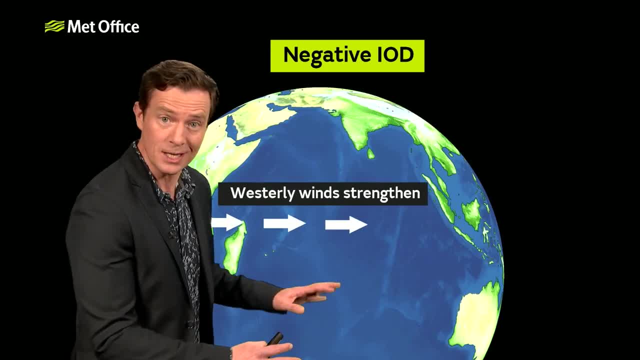